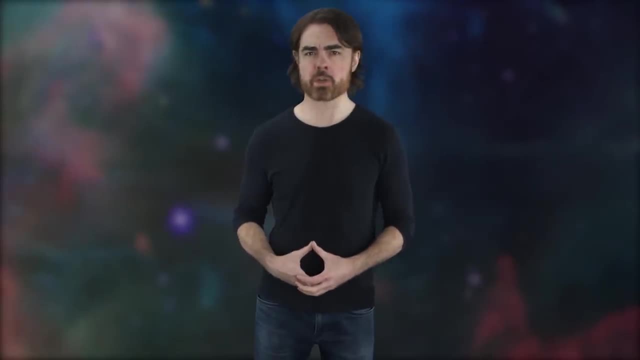 be on the verge of tackling things like Hawking radiation, But as you'll see today, in that unraveling we are led unavoidably to Heisenberg's uncertainty principle. The uncertainty principle is most often expressed in terms of position and momentum. We cannot simultaneously know both position and momentum for a quantum system with absolute precision. Try to perfectly nail down a particle's position and we have complete uncertainty about its momentum. And it's not just because our measurement of position requires us to interact with the particle, therefore changing. 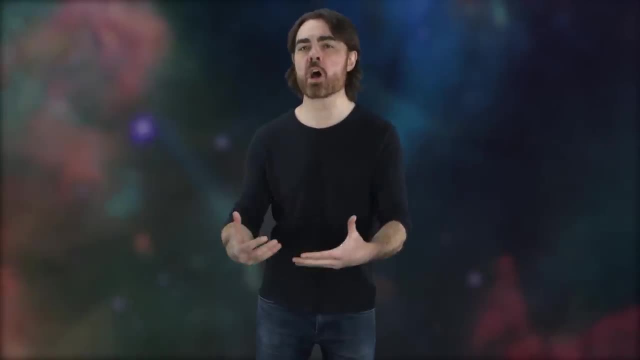 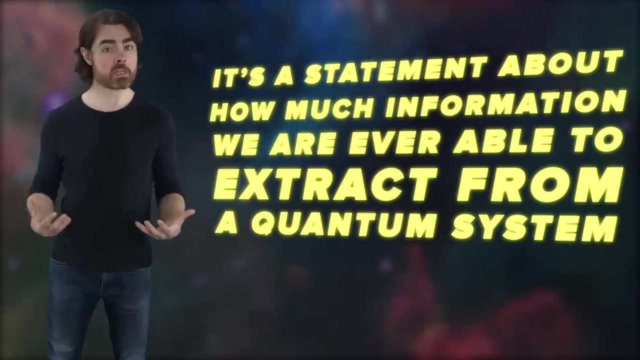 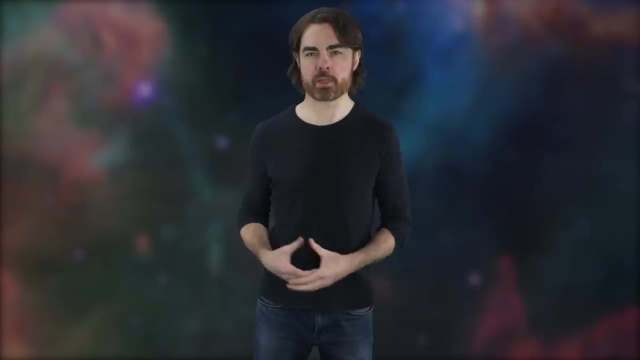 its momentum. No, the uncertainty principle exists alongside this observer effect. It's instead a statement about how much information we are ever able to extract from a quantum system. To understand the origin of the uncertainty principle, we don't need to know any quantum mechanics. 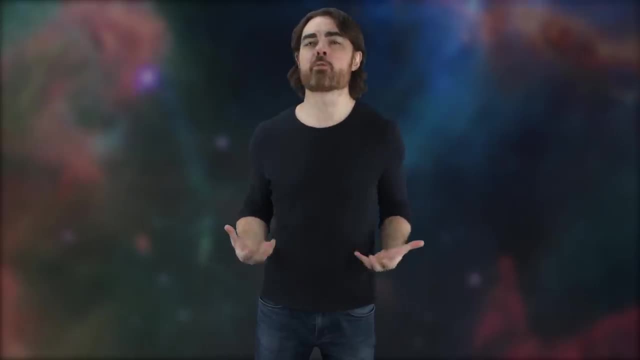 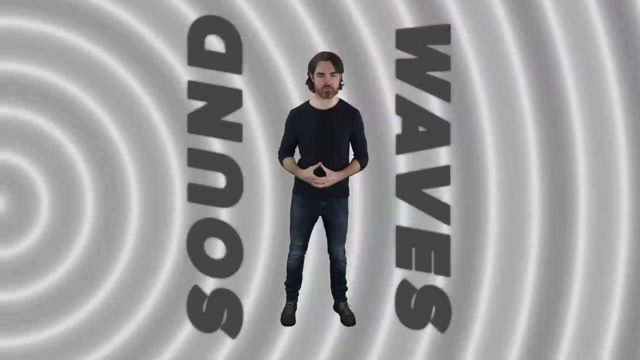 at least not to start with. See, quantum mechanics is a type of wave mechanics, a very weird type. However, it turns out that something like the uncertainty principle arises in any wave mechanics, So let's choose a type of wave that's a little more intuitive sound waves. 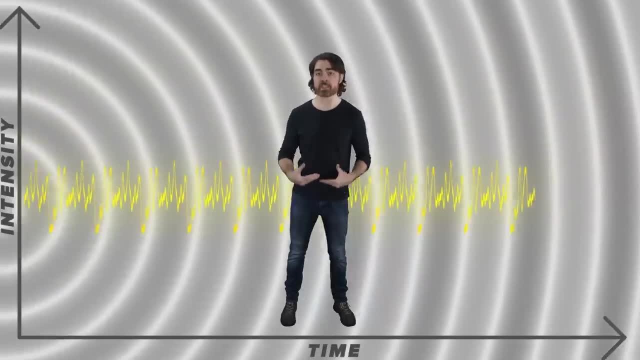 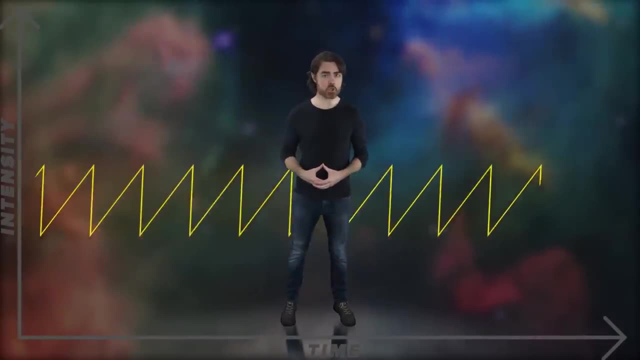 You can describe a sound wave just as the intensity of the wave as it passes by, so intensity changing over time, It can take really any shape. That shape determines what the wave sounds like to our ears. The sound wave for a simple, pure tone like a middle C. 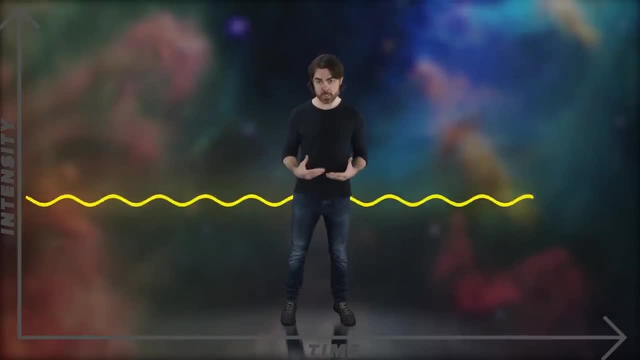 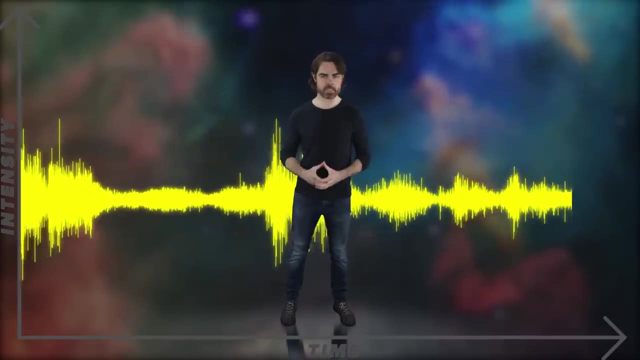 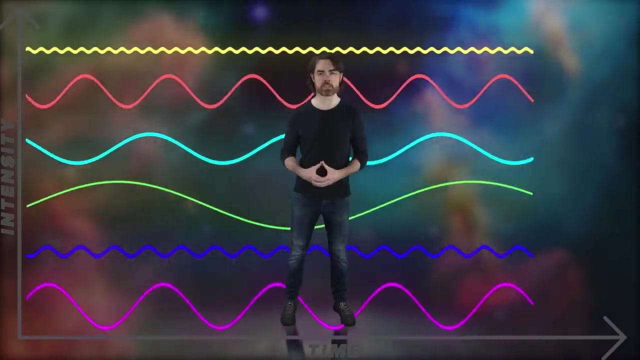 is a sinusoidal wave with the frequency determining the pitch of the tone. The sound wave from, say, an orchestra is extremely complex, But amazingly it can always be broken down into a combination of many simple sine waves of different frequencies. This is Fourier's theorem, after French mathematician Jean-Baptiste. 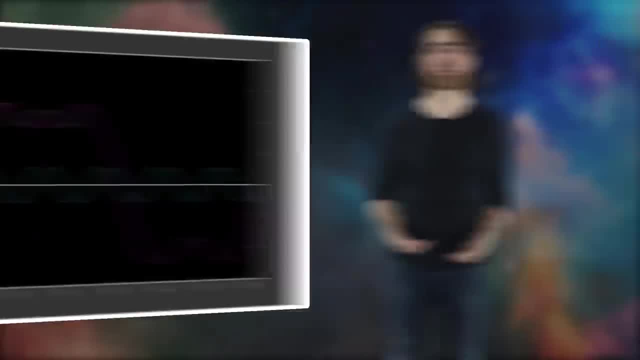 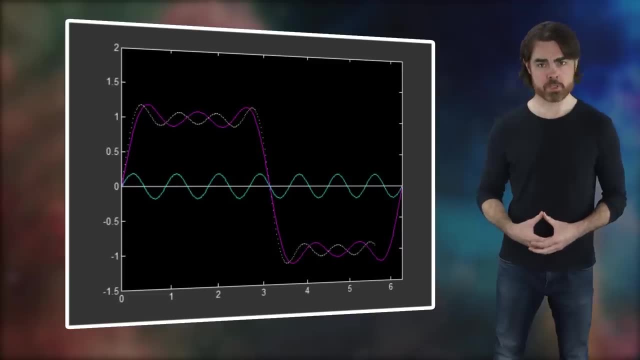 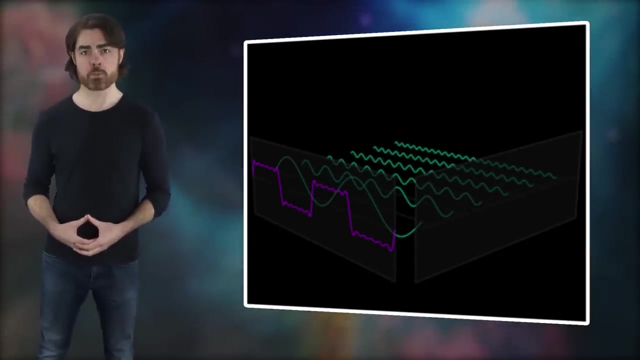 Joseph Fourier. It states that any complex sound wave can be decomposed into a number of sine waves, The sine waves of different frequencies, each with a different strength, stacked on top of each other or superposed. In fact, instead of representing a sound wave in terms, 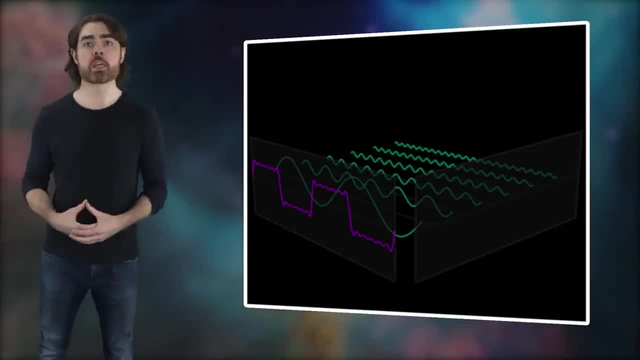 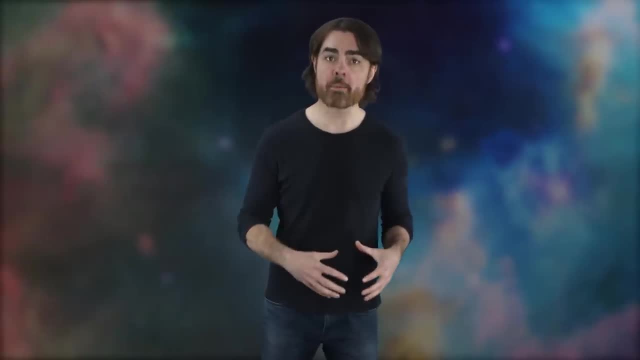 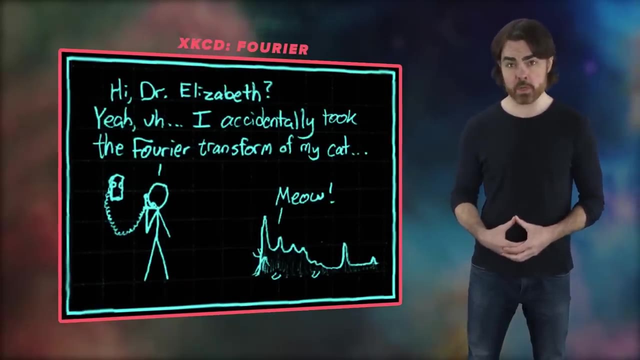 of intensity changing with time. you can also represent it in terms of its frequency components, each with its own weighting or strength. When you switch between a time and a frequency representation, you're doing a Fourier: transform In fact. digital audio equipment stores manipulates. 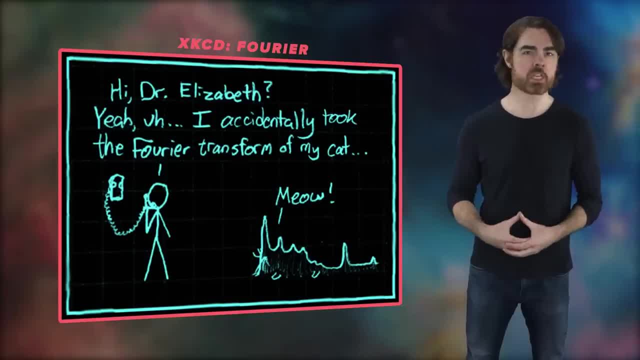 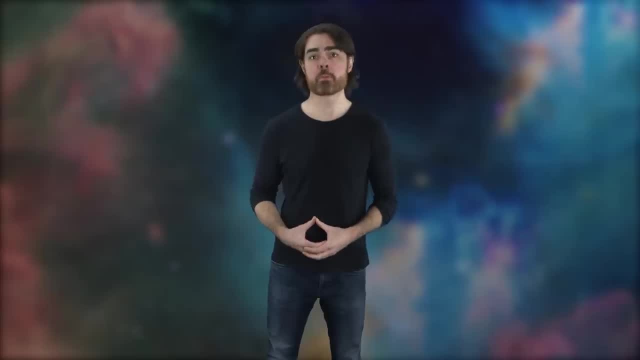 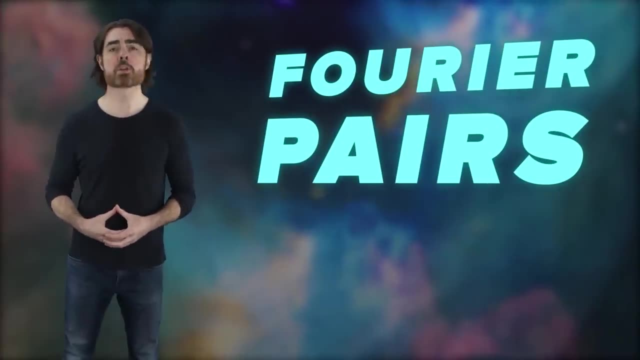 and transmits sound in its frequency. representation In the physics of sound, time and frequency have a special relationship because any sound wave can be represented in terms of one or the other. We call them Fourier pairs, also sometimes conjugate variables. OK, so we can make any shape sound wave. 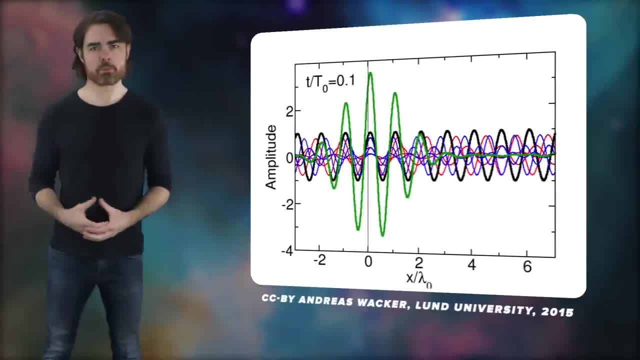 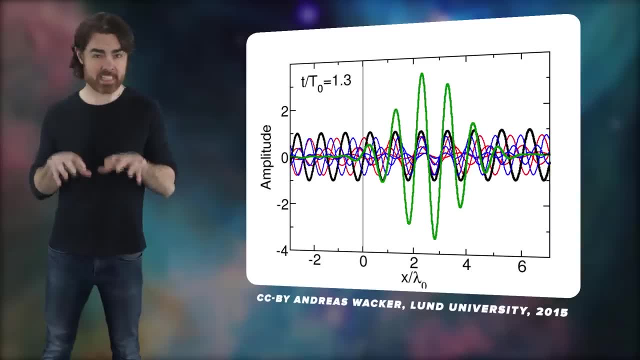 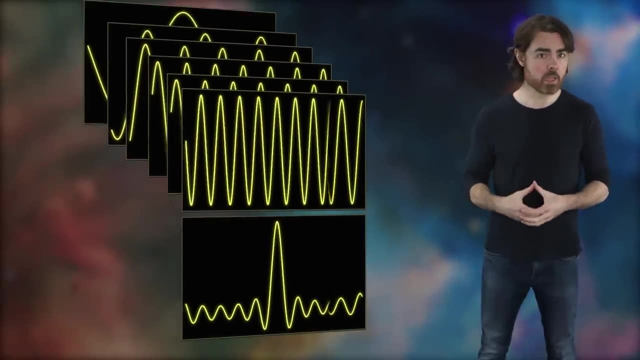 with a series of sine waves of different frequencies. For example, you can build a wave packet by adding frequency components with the right phases to destructively interfere everywhere except within a small region. The tighter you want to make that time window for the wave packet, the more frequency components you need to use. 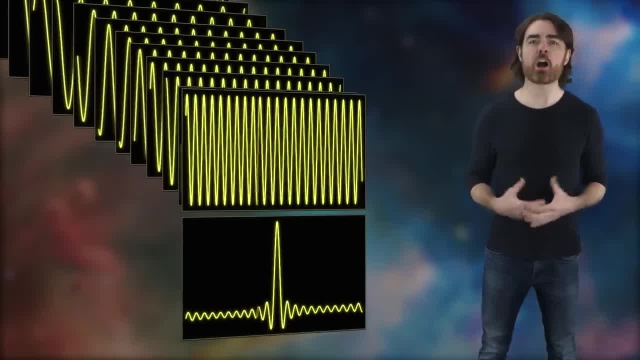 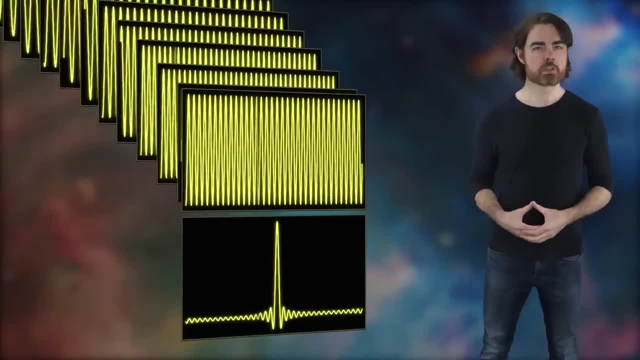 In fact, to get those steep edges of the wave packet, you need to add higher and higher frequencies, because the high frequency components are the ones that give you rapid changes in intensity. So what if you try to compress the wave packet to a single spike, a blip of sound? 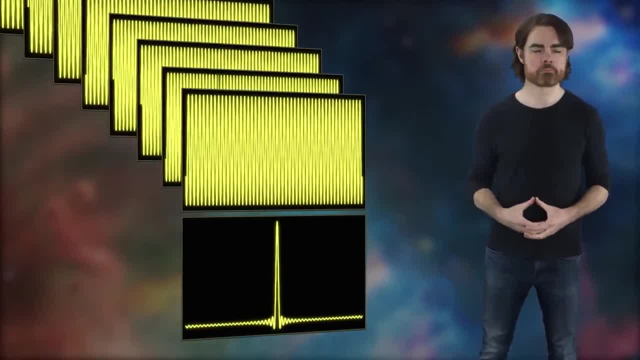 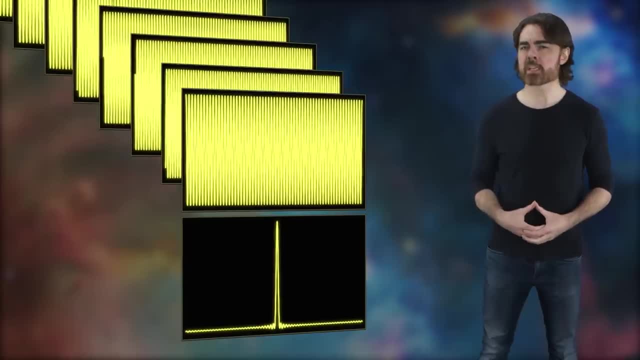 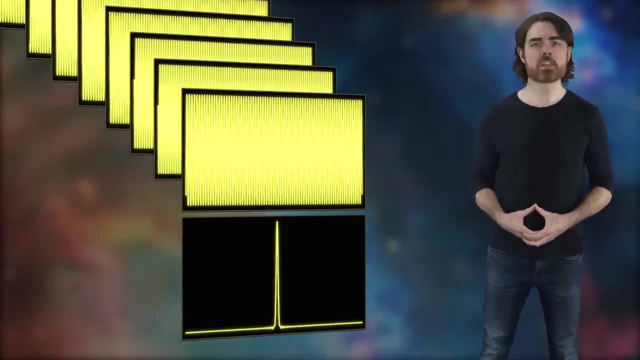 that exists for only one instant in time. Is it even possible to make an instantaneous spike at one point in time out of a bunch of sine waves that themselves extend infinitely through time? In fact, it is, However, to get a spike at one point in time. 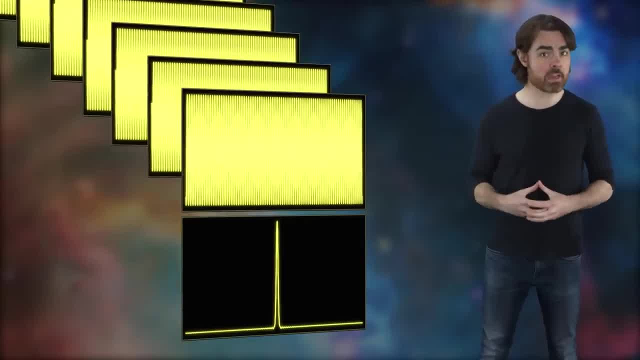 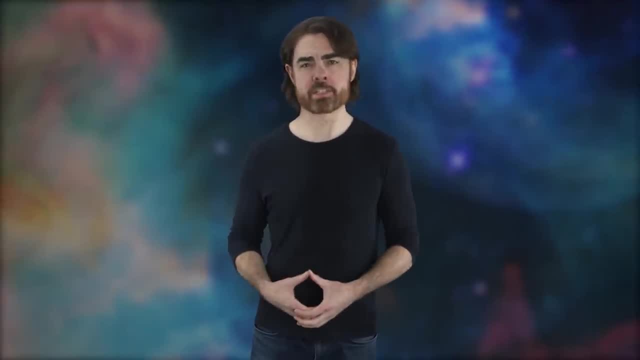 you need to use infinitely many different frequency sine waves, each of which exists at all points in time. So then, if we make a sound that is perfectly located in time, it doesn't have time, It doesn't have a frequency or it has all frequencies. 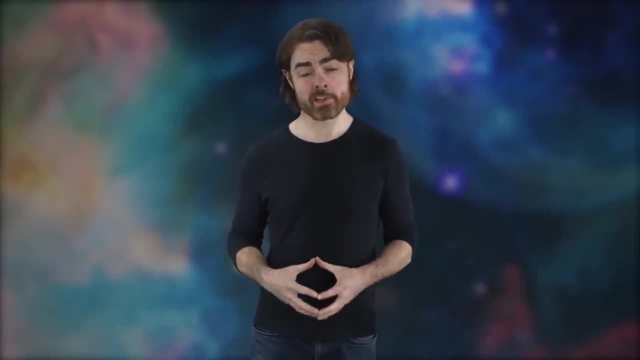 At the same time, a sound wave with a perfectly known frequency is a simple traveling sine wave that extends infinitely in time, so the time of its existence is undefined. That sounds an awful lot like a frequency time uncertainty principle for sound waves. Now, it's not really a statement about the fundamental. 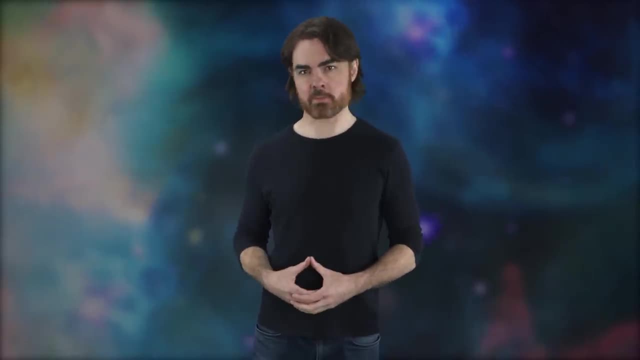 knowability of a sound wave, as is Heisenberg's uncertainty principle. It's more a statement about the sampling of frequencies needed to produce a given wave packet, But the underlying idea is the same. So how does this relate to the quantum world? 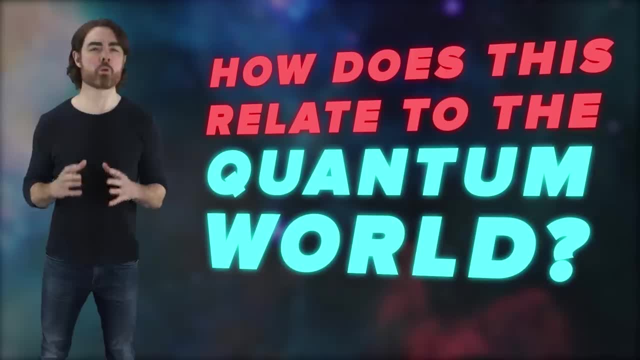 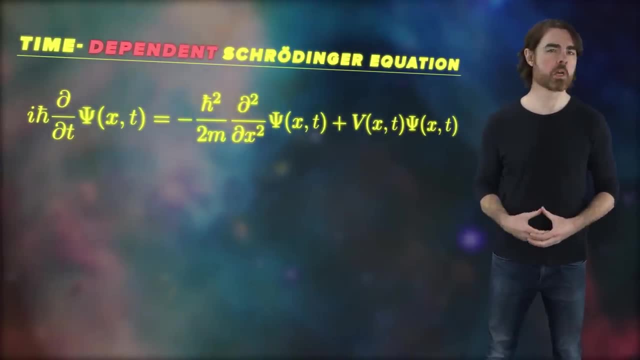 Well, before we get back to quantum fields, let's think about the wave function, the solution to the Schrodinger equation that contains all of the information about a quantum system. Like the sound wave, it oscillates through space at a particular frequency. 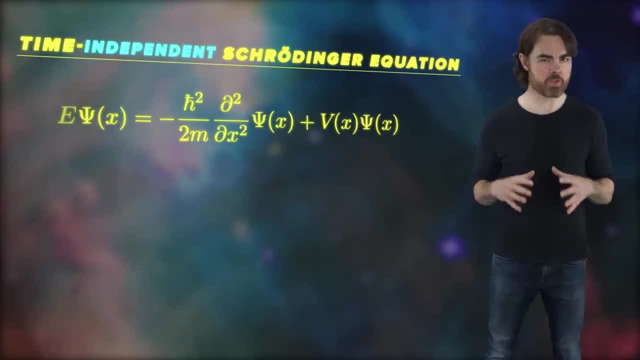 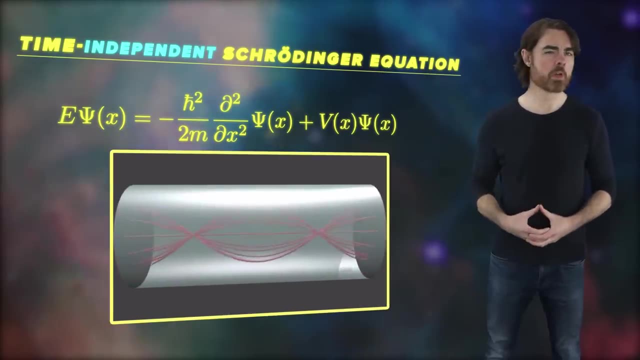 To keep things simple, we're just going to consider a wave function that doesn't vary in time. It only changes with position in space. This is more like a standing sound wave inside an organ pipe rather than the traveling sound wave from earlier. So position rather than time becomes. 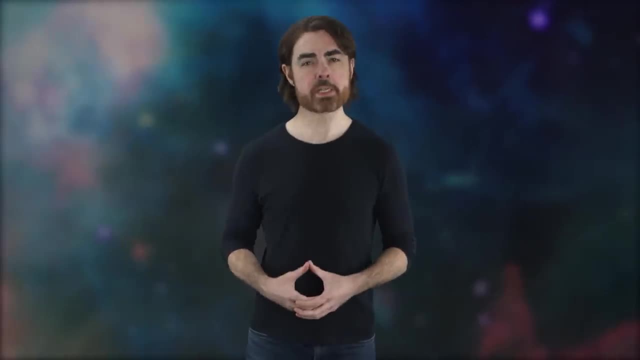 the first of our Fourier pair. The second of this pair is momentum, not frequency, See. momentum is sort of the generalization of frequency for what we call a matter wave. In the early days of quantum mechanics it was realized that photons are electromagnetic wave. 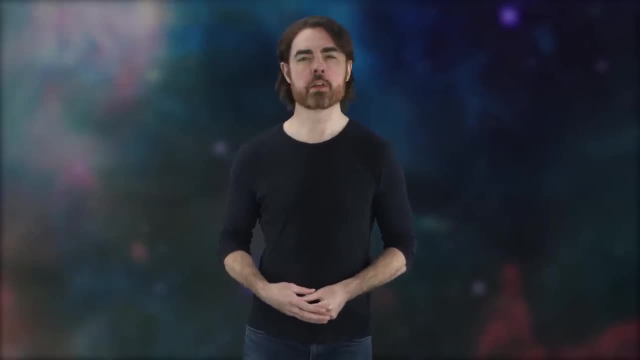 packets whose momentum is given by a wave. So it's not a matter wave, It's a quantum wave. So how do you deal with a chess situation? Well, the real question is as follows: We read time as momentum and it's parameter wave. 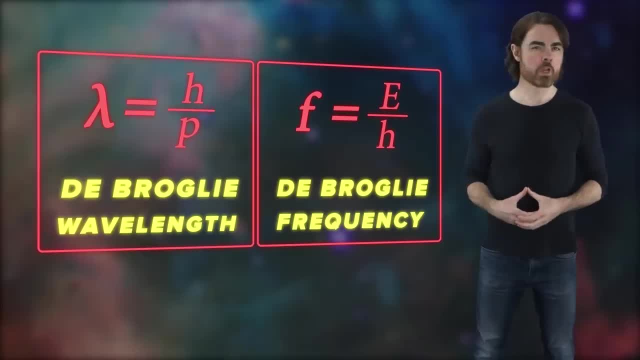 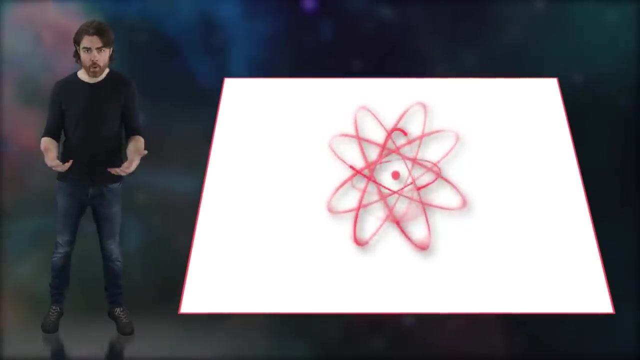 What is quantum motion? So our summation of time is the maximum Report that we're given when we say your sum of time is the level of momentum and time in Game 1. If you're doing quantum or you write down, each person that's. 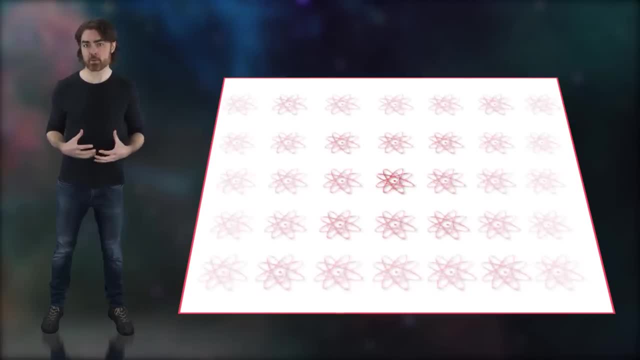 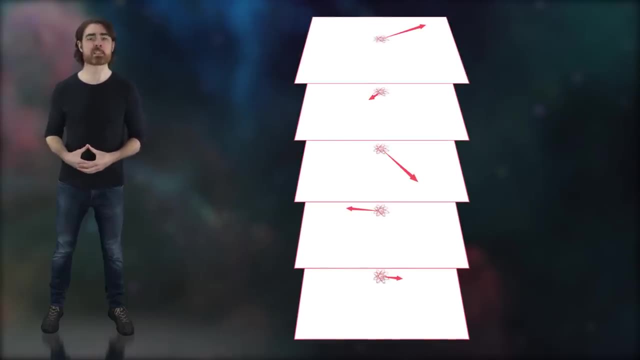 with accompanying intensities. think of it as the particle being smeared over possible positions, or as a combination of many momenta with accompanying intensities, in which case the particle would be smeared in momentum space, And of course this means that position and momentum 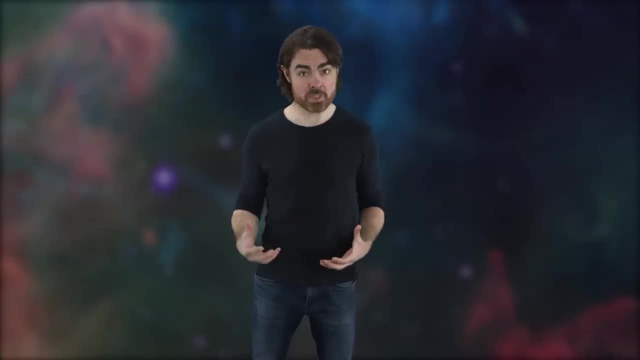 have the same kind of uncertainty relation that time and frequency had in the sound wave. But what does it even mean for a particle to be comprised of waves of many different positions or momenta? To answer this we need one more bit of physics. 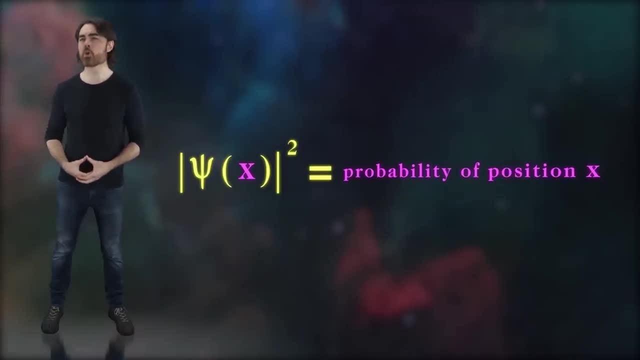 the interpretation of the wave function itself, known as the Born rule. The magnitude of the wave function squared is the probability distribution for the particle. If we're expressing the wave function in terms of position, then applying the Born rule tells us how likely we are to find the particle at any given point. 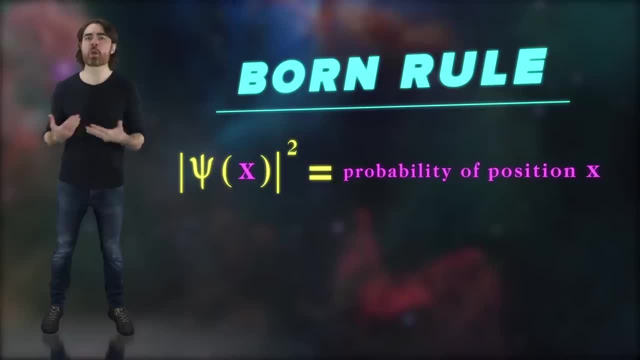 when we make a measurement, Or put another way, the range of positions in which the particle is likely to be located. were we to look, If we apply the Born rule to the momentum wave function, then we learn the range of momenta the particle is likely to have. 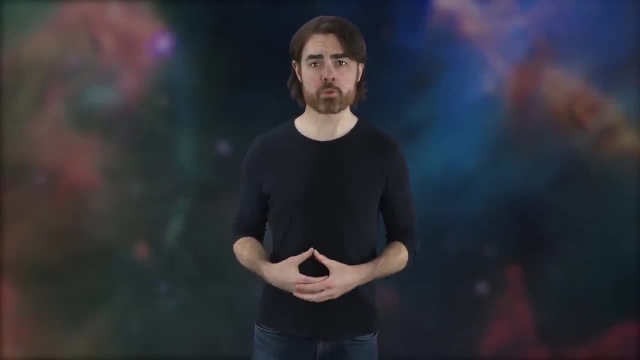 So if we measure a particle's position, then from our point of view its wave function is highly localized in space. We know where the particle is. The resulting particle wave packet, now constrained in position, can only be described as a superposition of waves with a very large range. 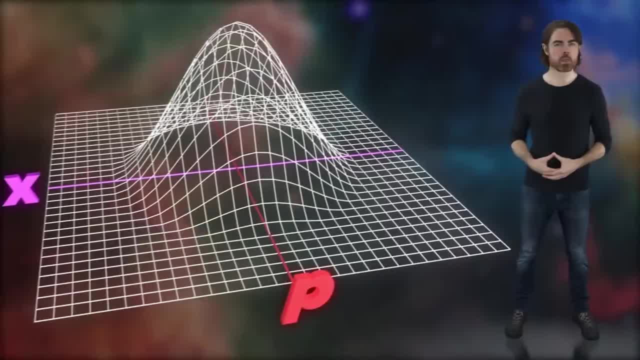 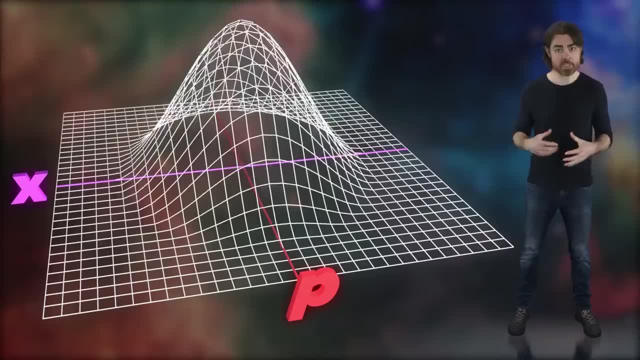 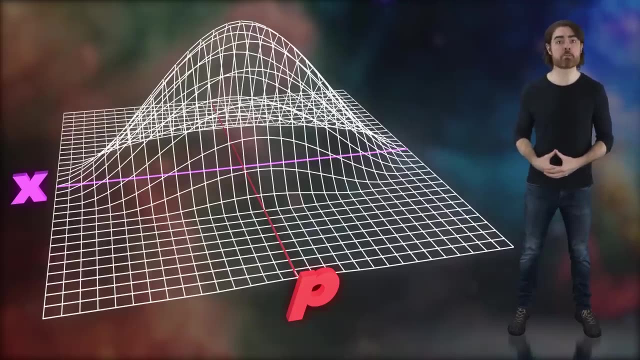 of different momenta via a Fourier transform. The result is a very fat momentum wave function that gives a wide range of possible momenta. The more precisely we try to measure position, the narrower we make its position wave function, and so the less certain we become about its momentum. 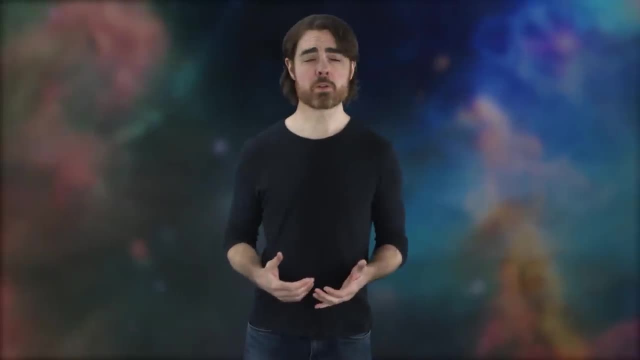 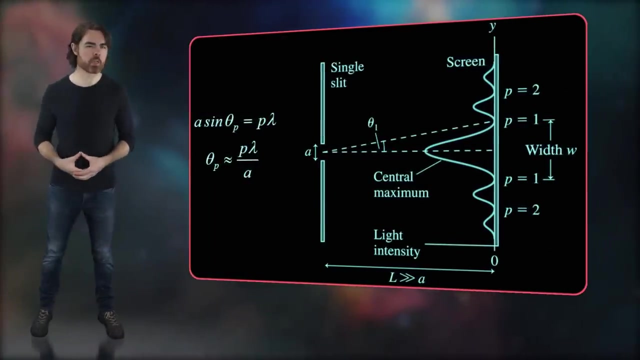 as that momentum wave function gets wider. This is all super abstract, but a concrete example is single slit diffraction. If we increase our certainty of the position of a particle by narrowing the slit, we also increase the uncertainty of its momentum as it passes the slit. 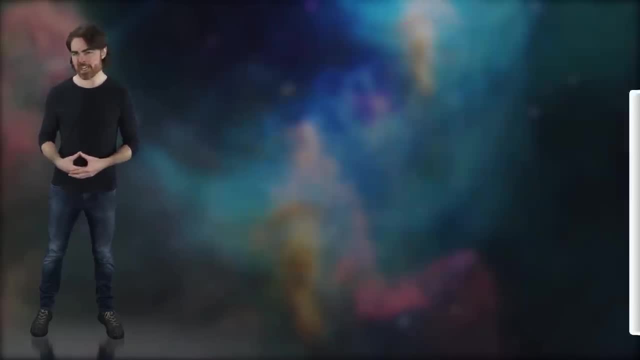 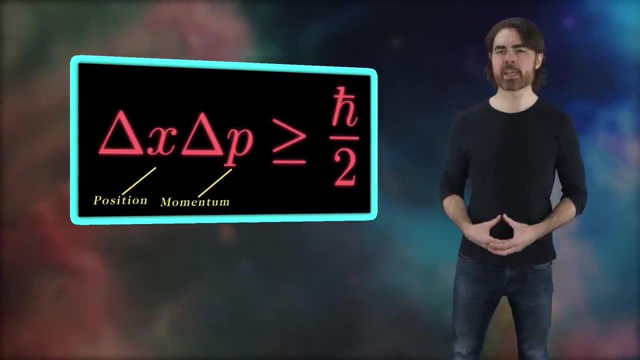 This results in an increasing spread in final locations. Check out Veritasium's excellent video to see this in action. So that's exactly the uncertainty principle. It's a statement about how much of a quantum system's information is accessible at a fundamental level. 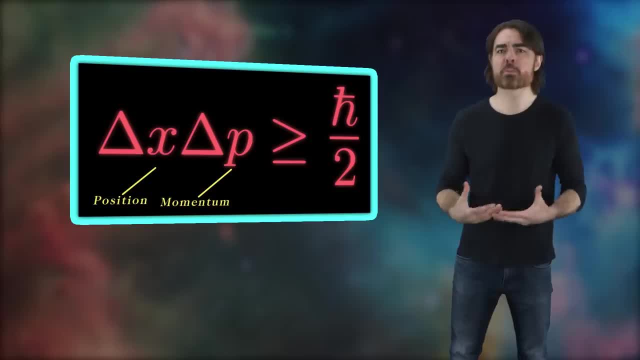 It's an unavoidable outcome of describing particles as the superposition of waves, waves that can be represented in terms of either position or momentum. The fact that both can't be known simultaneously with perfect precision is a property of the nature of the wave function itself. 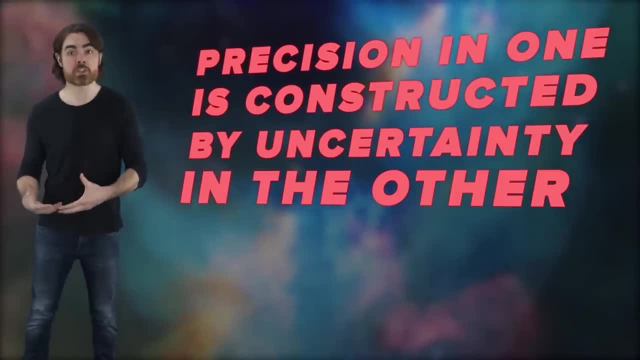 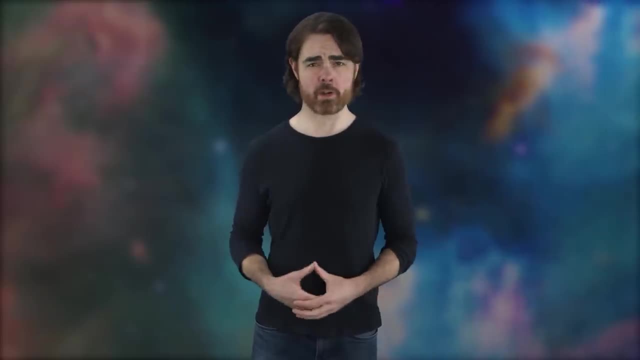 Precision in one is actually constructed by the uncertainty in the other. OK, so what does this old school quantum mechanics have to do with quantum field theory and Hawking radiation? Well, the key to understanding these things is to be able to switch between thinking. 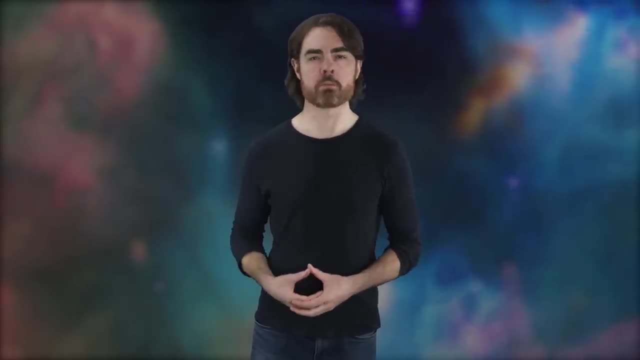 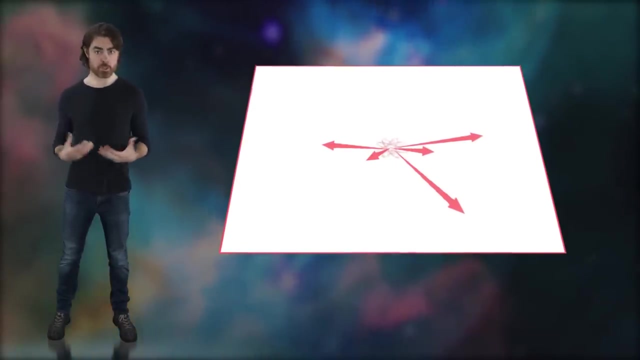 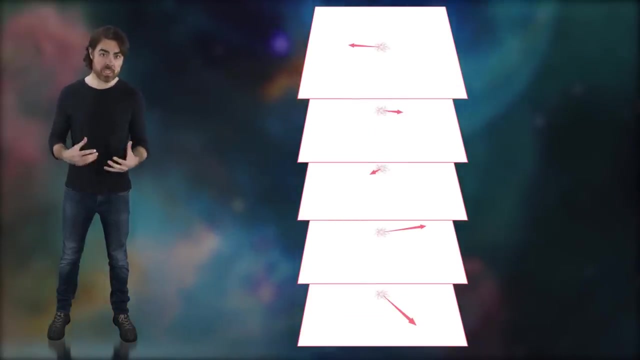 about quantum fields in terms of position versus momentum. See a single particle. a quantum field vibration perfectly localized at one spot in space can also be described as infinite oscillations in momentum space, spanning all possible momenta. But each of these oscillations in momentum space 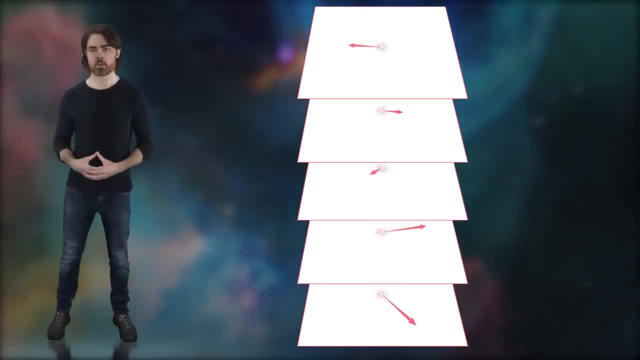 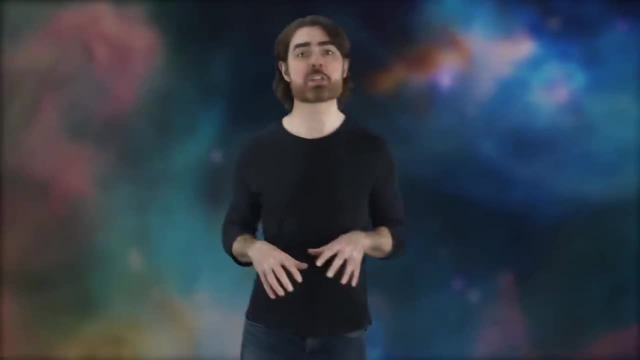 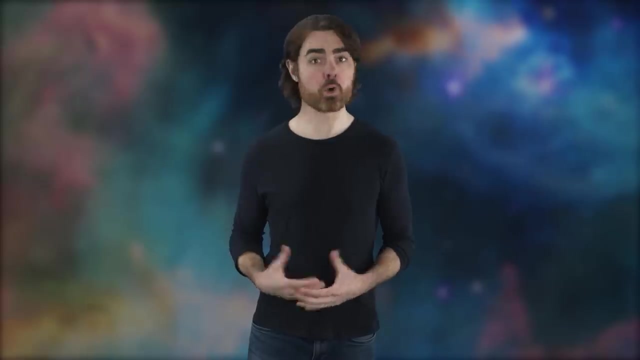 are equivalent to particles with highly specific momenta. The uncertainty principle therefore tells us that they must be completely unconstrained in position. So A perfectly spatially localized particle is equally an infinite number of momentum particles that themselves occupy all locations in the universe. 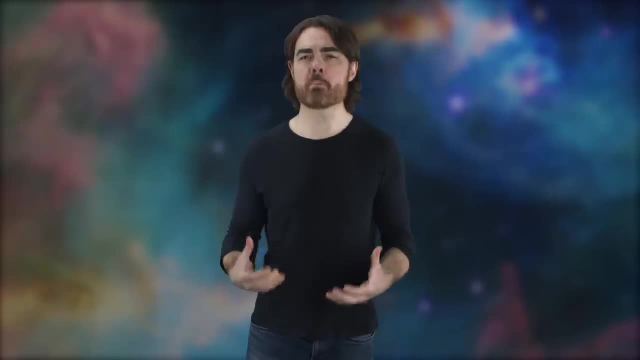 It's only by manipulating quantum fields in this strange momentum space, by adding and removing these spatially infinite particles, that we can describe how the quantum vacuum changes to give us phenomena like UNRWA and Hawking radiation, which you'll soon understand as some of the weirdest behaviors. 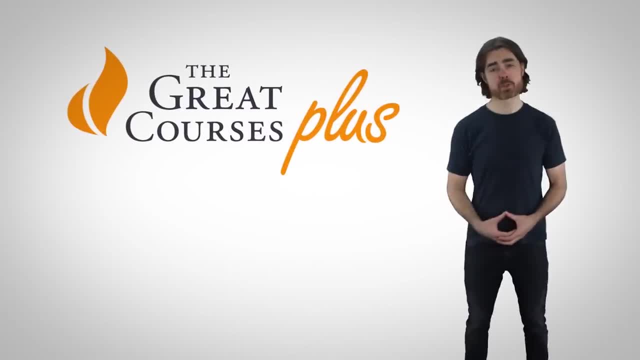 as well as some of the most bizarre phenomena that we've ever seen in the universe. Thanks to The Great Courses Plus for supporting PBS Digital Studios, The Great Courses Plus is a digital learning service that allows you to learn about a range of topics from Ivy League professors and other experts. 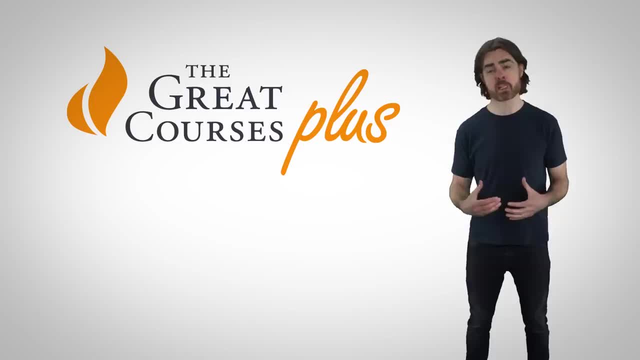 from around the world. Go to wwwthegreatcoursespluscom. slash spacetime and get access to a library of different video lectures about science, math, history, literature or even how to cook, play chess or become a photographer. New subjects, lectures and professors. 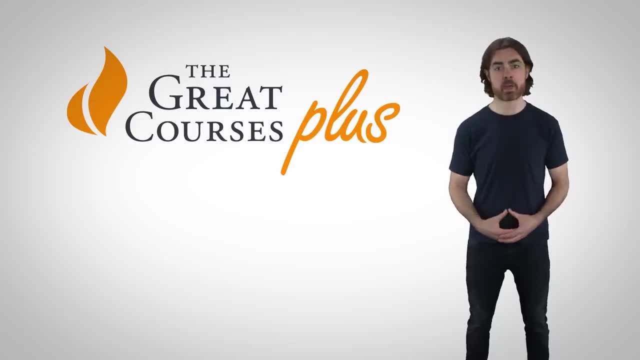 are added every month. Now our recent discussions about the quantum world are leading up to some pretty mind-blowing episodes. To help prep yourself even better, you could check out Benjamin Schumacher's series Quantum Mechanics, which includes a great episode. 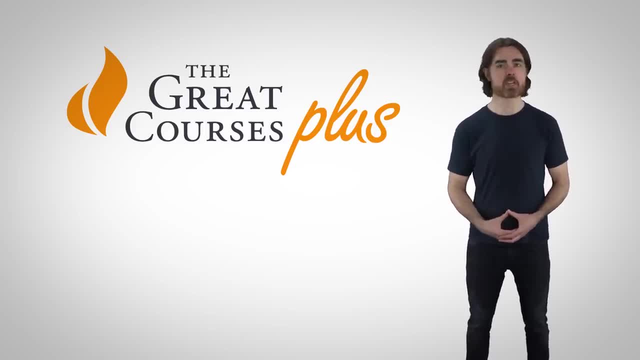 on the uncertainty principle. Help support the series and start your free one-month trial by clicking on the link below or going to thegreatcoursespluscom slash spacetime. OK, so I traveled a bit over the past two weeks and so we missed one of our comments. 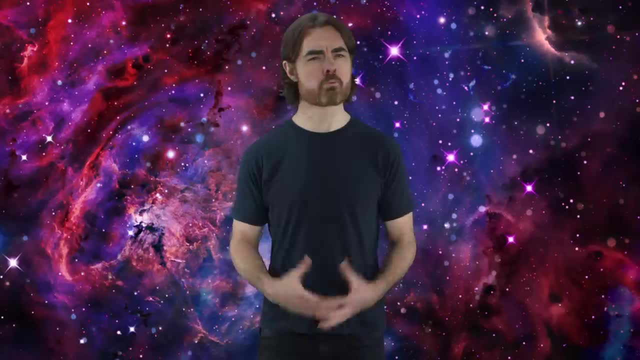 So I'm going to give you a few quick comment responses. Today we're going to cover our episode on robots that sacrifice themselves for science, as well as our episode on citizen science. First, thanks to everyone who pointed out the editing error at the end of the suicide robots episode. 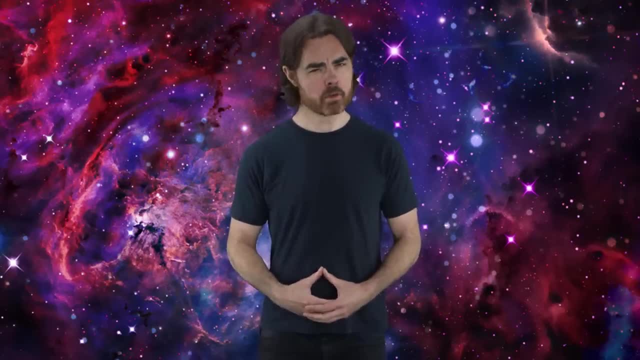 where we accidentally included both of the two takes of the last line. Totally unintentional, but hey, it was a pretty good line, right? Also thanks to everyone who noticed my mispronunciation of Enceladus. You know those words? you've never.